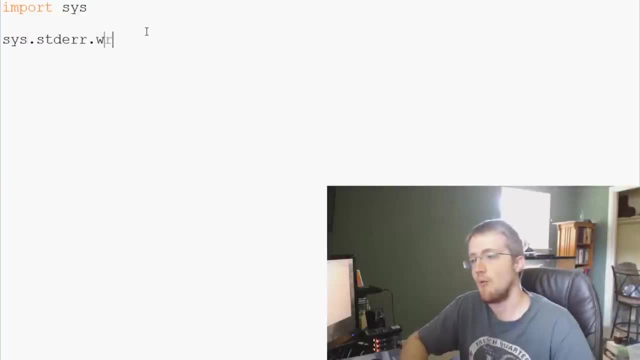 So first let's go ahead and type Sysstdarwrite, and we're just going to write test, And after you do S-E-E-R, it's a good idea to go ahead and do Sysstdarflush. So we'll say test, So we print this out and you should get output like this, So that red error text that you're used to seeing. if you've ever gotten an error- which I'm sure you have And I'm going to change this to- this- is S-E-E-R. 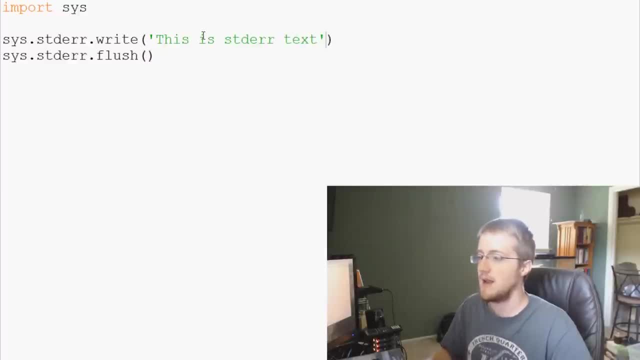 S-E-E-R, S-E-E-R, S-E-E-R, S-E-E-R, S-E-E-R, S-E-E-R, STD error text, like that. and then I'll show you guys, now sysstdoutwrite, and then we'll say: this is SC out text. and also what you're gonna see is that 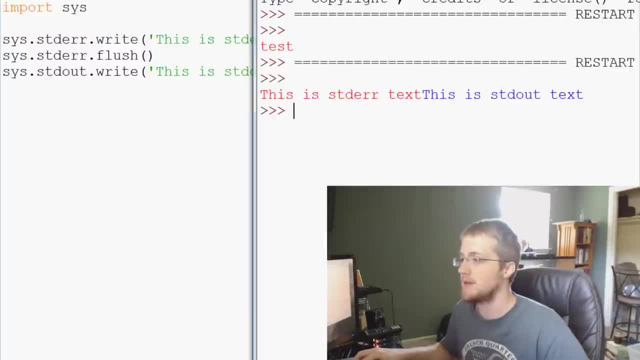 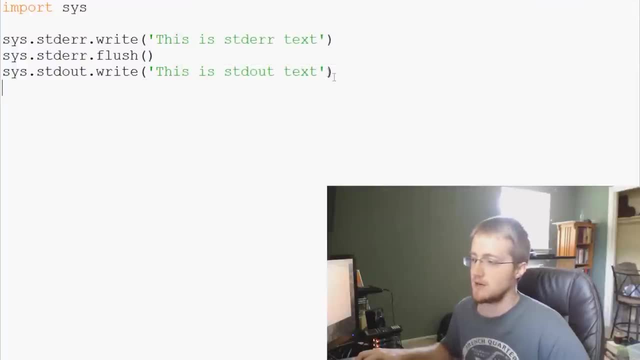 I'll show you guys in a second. so we'll save and run that and you get this. so you get this error text and then I see out text is just that blue text. but you see they're on the same line. so what we can do is at the end of all of these you 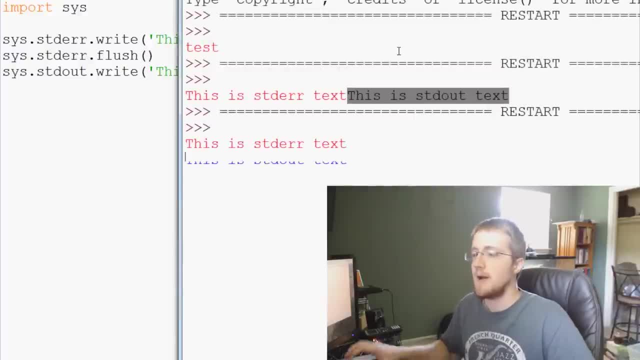 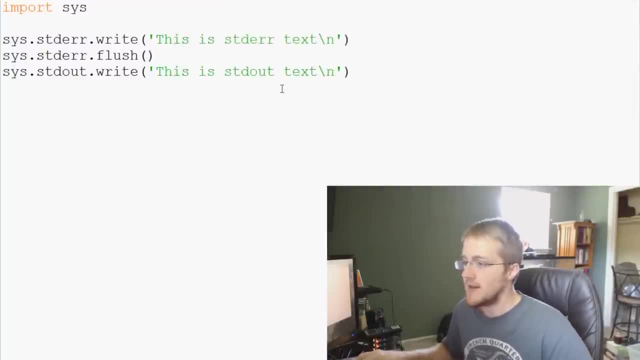 would all kind of want to always add a new line there. that way everything continues on on the next line. so it just kind of organizes it a little bit for you guys. so, anyway, close out of that, and now we get to the fun stuff. this is argv. 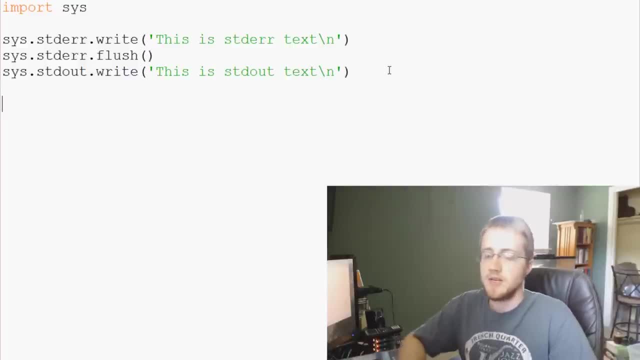 so just to show you guys a basic example, we could say: print sysargv like this, and if we print that, we get basically the file path, and this is the path to the file I'm editing right now. it's just template dot pi. now that, basically, is just gonna give you the file name. okay, but what we can. 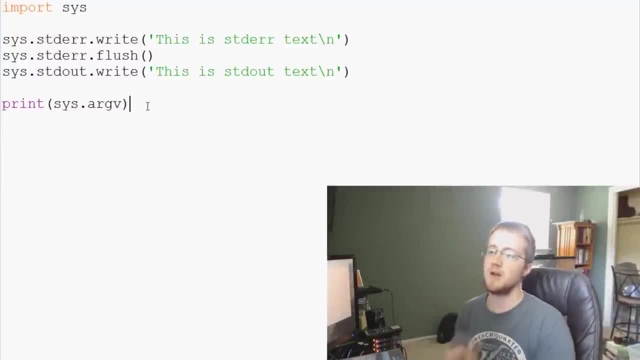 do with this is actually pretty cool. we can pass arguments into this Python file using our command line, which means using any other language, basically, or you can use the command line yourself as well, but you can use it for, like batch scripts, all kinds of really really cool stuff. so, anyway, or a really communication. 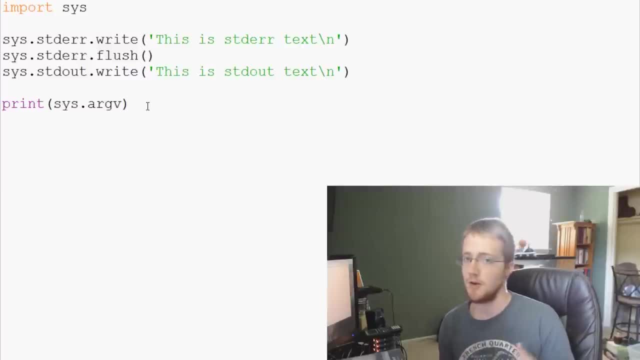 between PHP and Python or Perl or Ruby or whatever language. you're trying to use this to communicate back and forth, and, anyway, let's go ahead and get started. so sysargv is just gonna display all of the arguments, so what I can do here, though, is we'll save this, and, in fact, let me do something over here. let's. 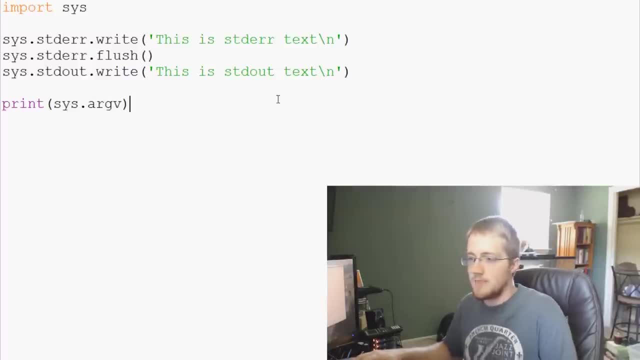 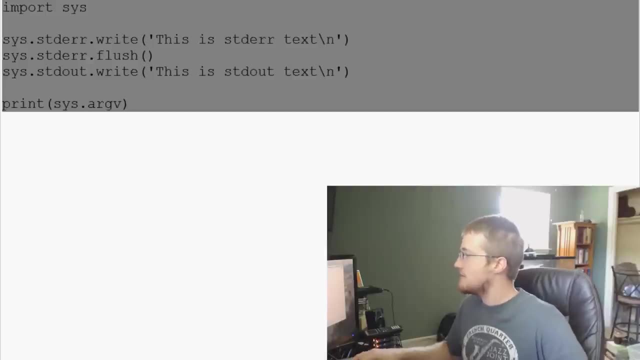 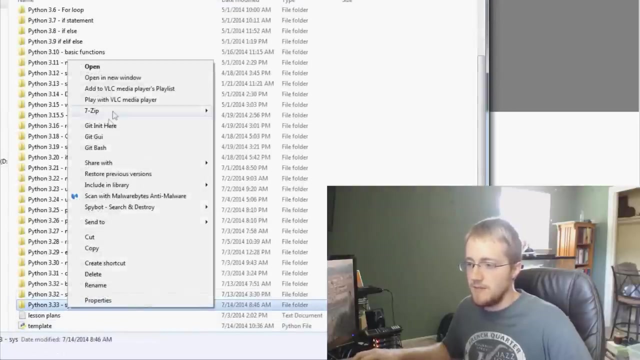 bring this. let's just copy and paste this into this file save. so I've saved that this data to this file here. that's in sys and we'll. so we'll come over here. we have sys and if you hold your shift key and right-click on the folder here, 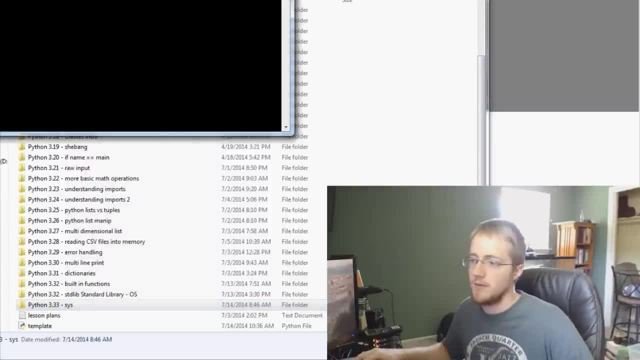 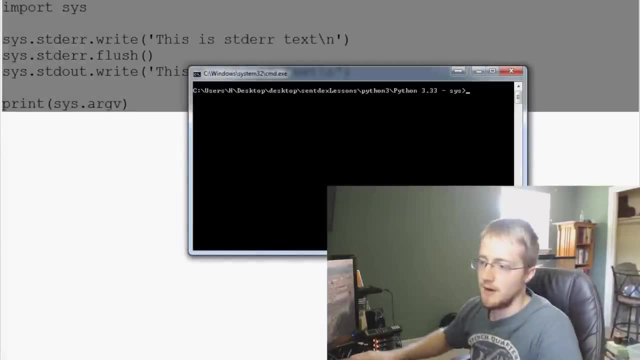 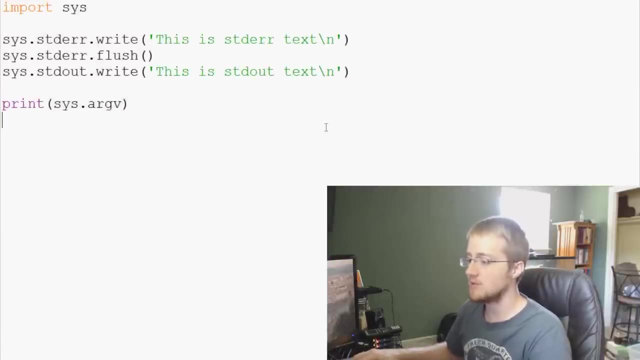 that you're in. you can open the command line there if you're on Windows. anyway, I'm not sure if it works on Linux or not, but you can on Windows, and so now we've opened up this file that looks just like this. okay, and in fact, mmm, I guess we'll. 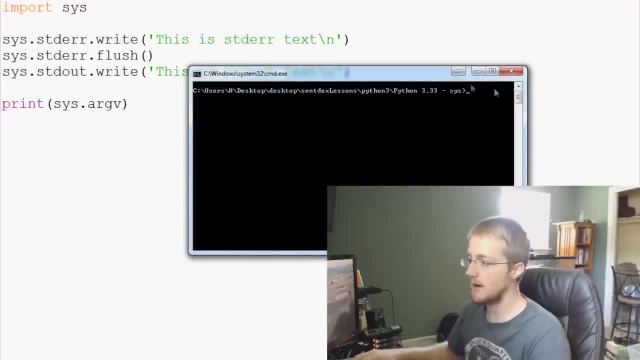 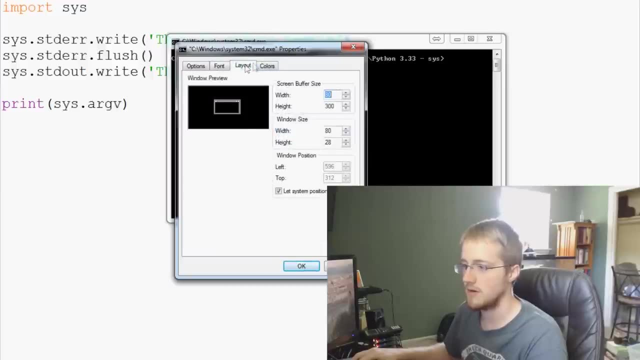 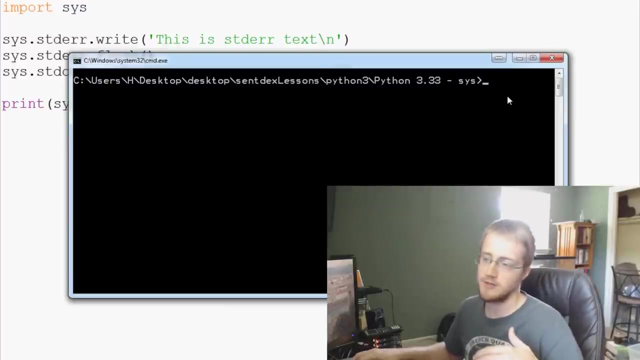 leave that input output text just for kicks for now. so let me see if I can make this a little bigger for you guys. just change the font size. wow, okay, I guess we'll just stick with this for now. so in here, now we can start passing arguments through here. so what we can do. 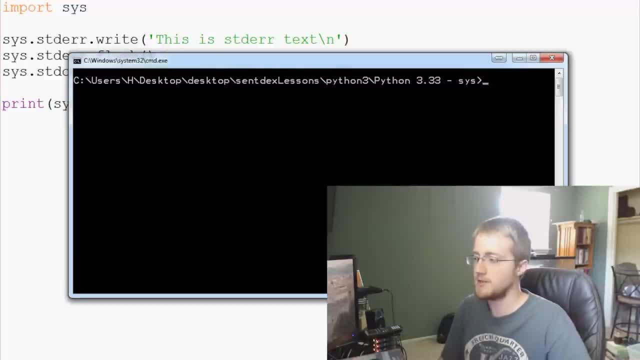 is. I've changed the file name to assist up high. so if I run the program and then if I hit enter, I'm gonna see that the system is just not Python syspy like that. It's going to give us our st-airtext, st-outtext. 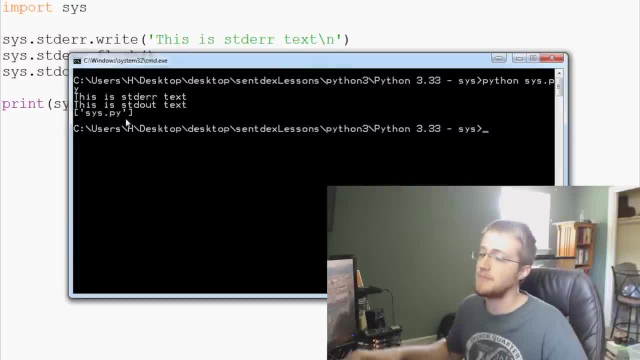 and then it's giving us our argv And our argv is just that file name that we just ran through. So argv is basically all the arguments that you pass through Python. So when we ran Python, our first argument really was that file name syspy right. 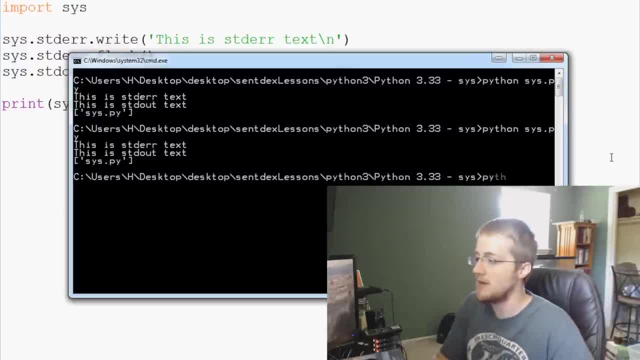 So that's why we get syspy. But we can pass other things through, So we can say: python, syspy, look at that, Run that. and now we get this Python list of syspy and then look at that. Now what I want to do is let's come back over to Python 3, sys. 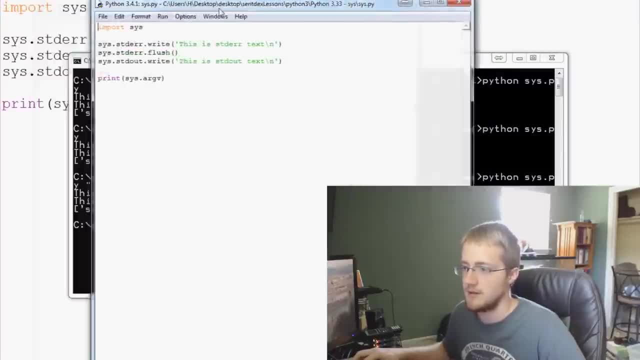 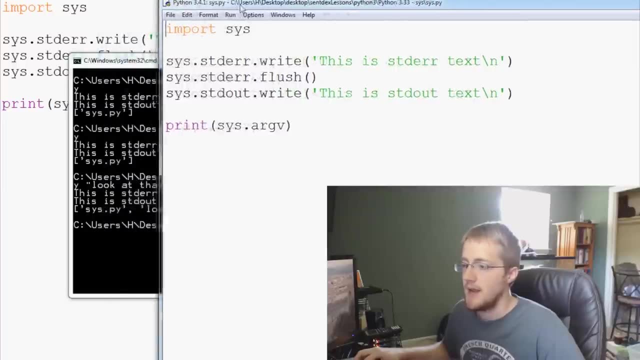 We'll open that up, and this is the one that we just made. So this is the data that's in this file, And let me go ahead and make this big text too. so it's good to see And see this is true. 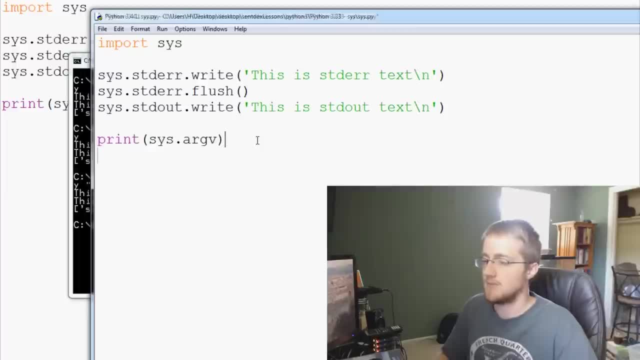 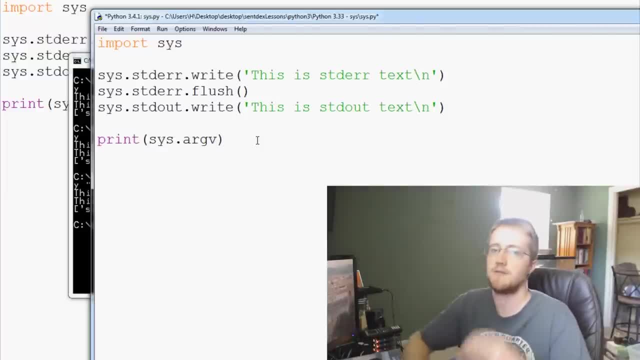 before you start referencing the arguments. it's a good idea to go ahead and make a check for that amount of arguments. So here let's say we're just going to have the file name and then one more argument that we're expecting. So we're going to say: if len sysargv. 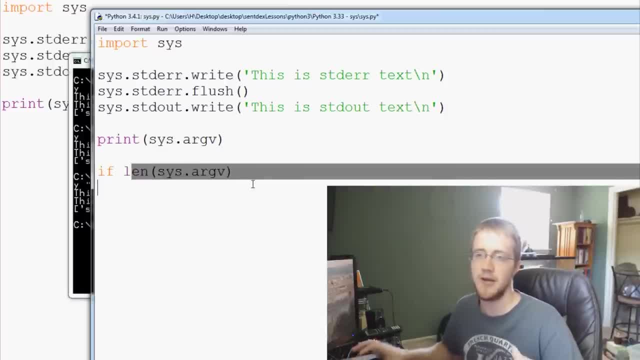 and what this does is it just tells us the length of a list. So if you had 15 elements, len sister RV would be 15, right? so if the length of sista RV is greater than 1- so we have more than one argument- then what we want to do is let's go ahead and just 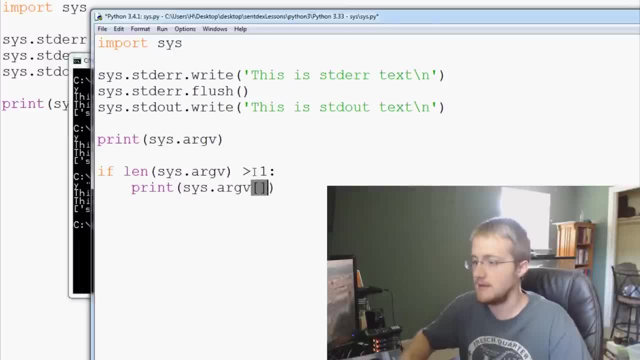 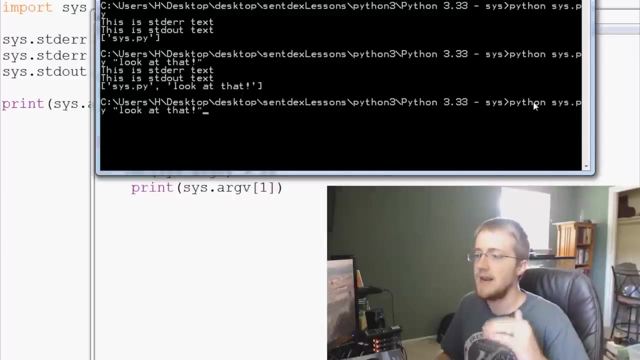 print sista RV and then one. so this one, right, the first element is zero, the second element is called one. it has an idea one. so we'll save that and we'll come back over here and we're going to do up arrow. look at that. and now what? 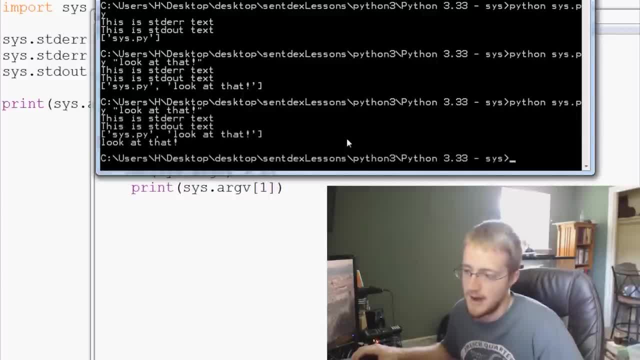 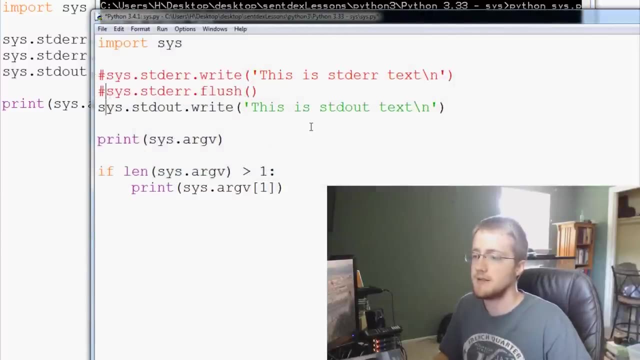 it's going to do is you see how it printed out for us? you know that's the error and out, and then it prints us the list, but then we can. we can see here that we were able to actually reference. look at that specifically, because that was one of our argument variables. so now, just to keep things clean, let's come at 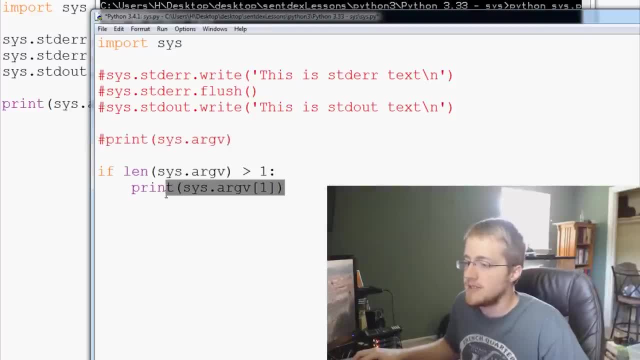 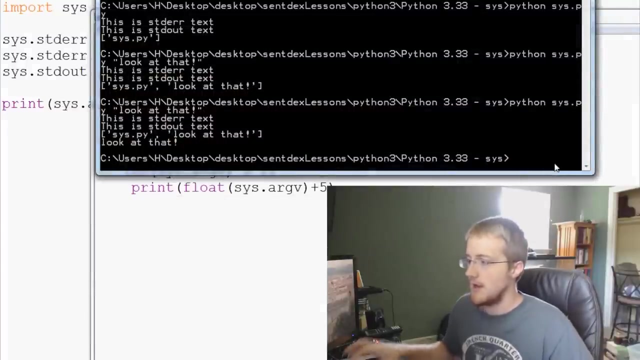 all this stuff out and this out, and now, instead of printing that, what we're going to say is: print in sista RV and actually let's do float just sista RV plus 5. can we get away with this? so we'll save that. come back over here and 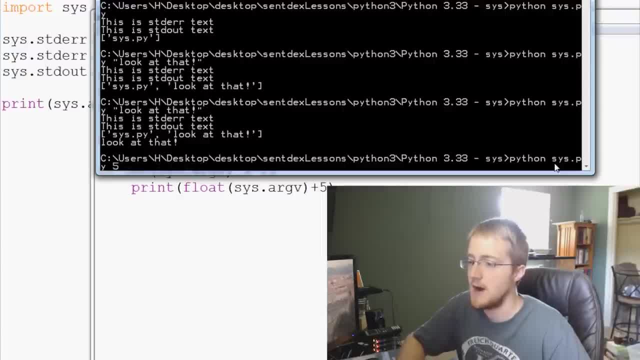 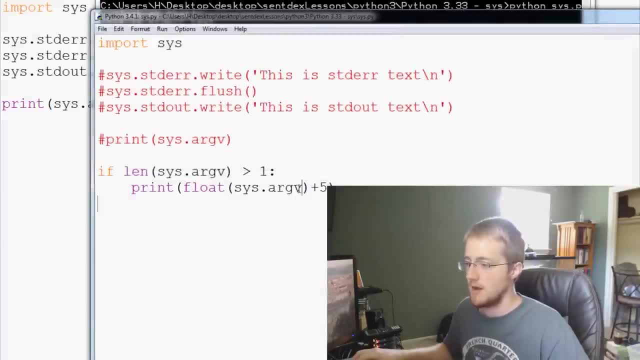 let's do instead of look at that. let's say 5, and so we can see that this must be a string or a number as the argument that we've passed through, um, and what we did here is we have to reference that. so let's try this one. 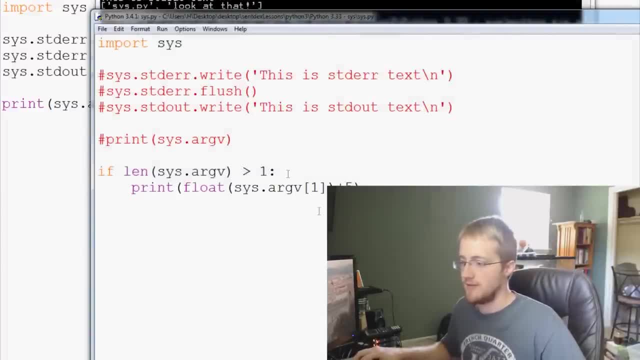 more time and now you get 10 point okay. so the reason why that had failed at first is we didn't put the the ID. so we're saying print float, the float version. now we could change this to in, and then it wouldn't be a float, but just. 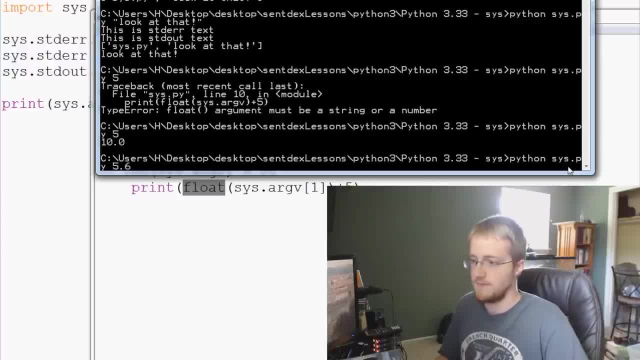 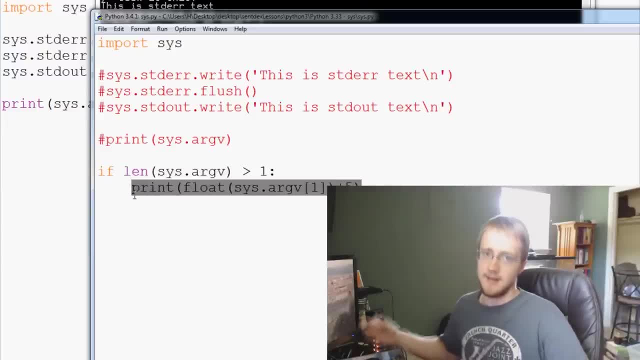 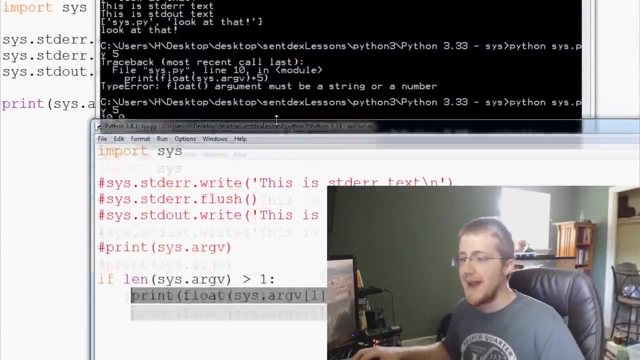 in case, like say you wanted to do five point six, seven or something like that, then it was ten point six seven because we added five. so we can start manipulating the values that come in into Python and so we can use this to pass values from anything right you can. 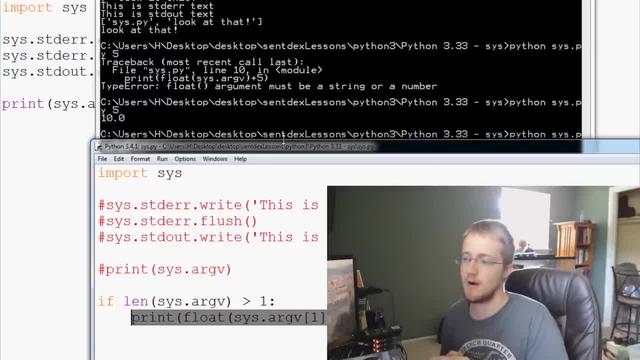 do it either from the command line itself. you can do you like. say you're writing something in PHP, like, for example: I use this kind of stuff to communicate between PHP and Python because I hate web design. I just hate it. i can't do it. and you said that you have a Django. 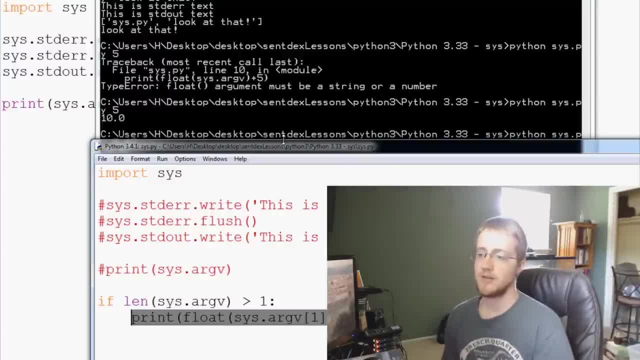 Anyway, I don't like doing it, and so most of the websites that I make for myself I just use WordPress, and WordPress is PHP, But for back-end stuff I use Python because Python is the language I know best. I don't really like PHP that much and I like Python. 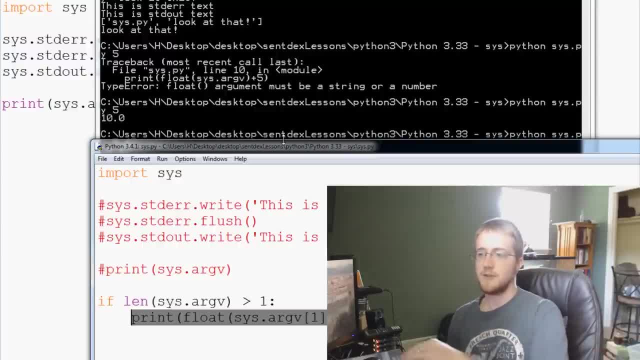 So what I'll do is I'll use this stuff to communicate between PHP and Python, which is otherwise kind of difficult to do. But you can use this to use Python. You can make a function and you can make that function argument, or the function parameter, rather a sysargument, right? 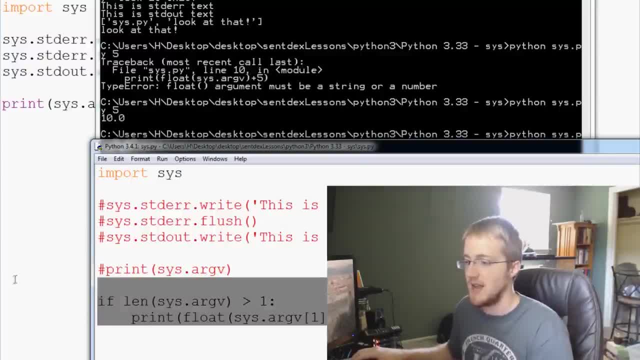 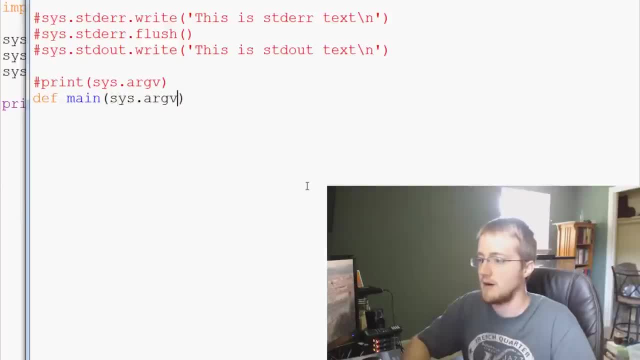 So for example, you could say import sys, and now we can come back up here and we can define main and then we can call it sysargv1, like that, And then We could say print sysargv1.. That's just our function, for example. 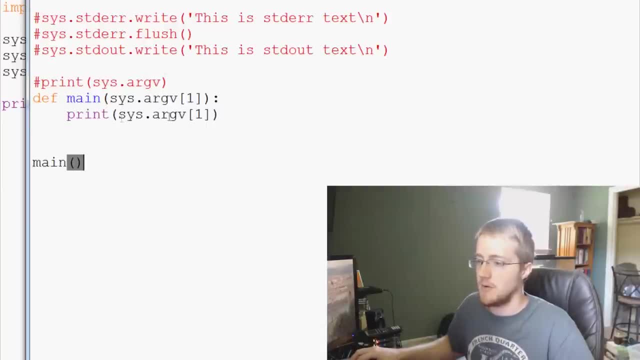 And then we go ahead and run main and really, actually, what we'd probably rather do is, instead of this, we'll just call it arg, and call this arg like that, Main sysargv1.. We can save that and we can come over to our command line here and do Python. 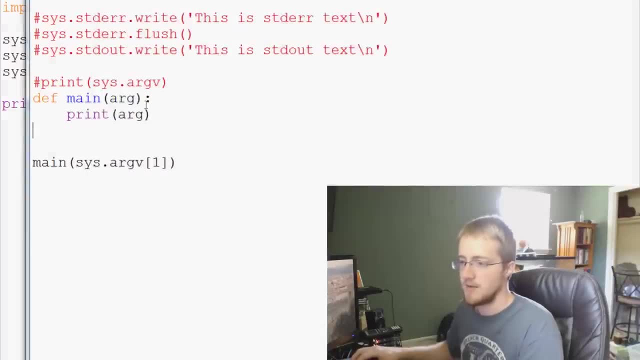 sysarg or syspy, rather 5.67.. We're going to print that argument in the main loop- We didn't save that yet- And run it and you can see here that we've commented out everything. We made this function that uses that argument.